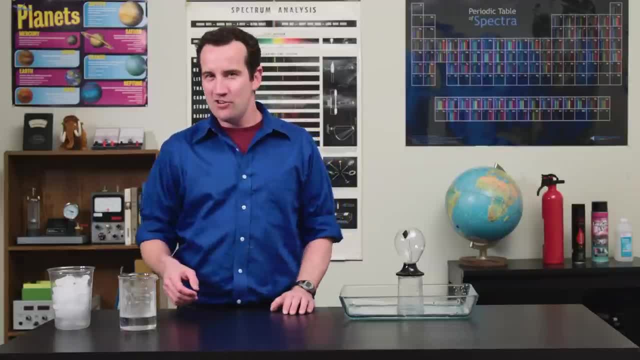 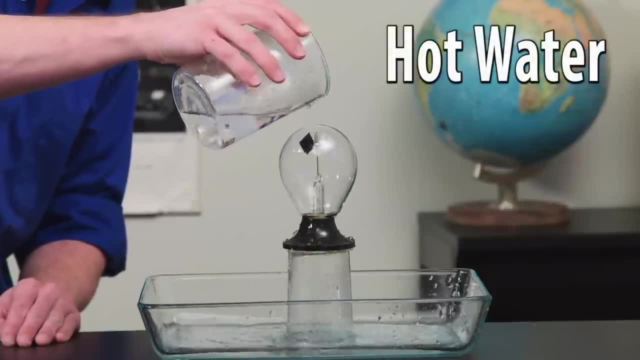 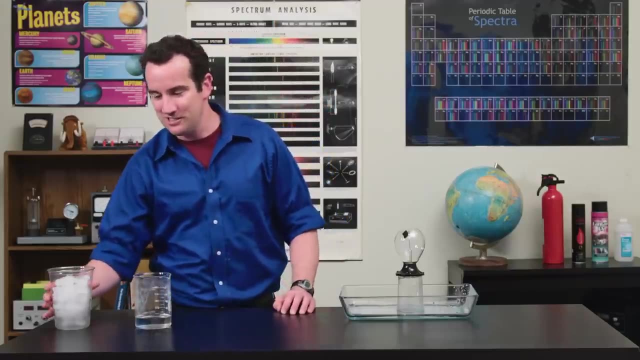 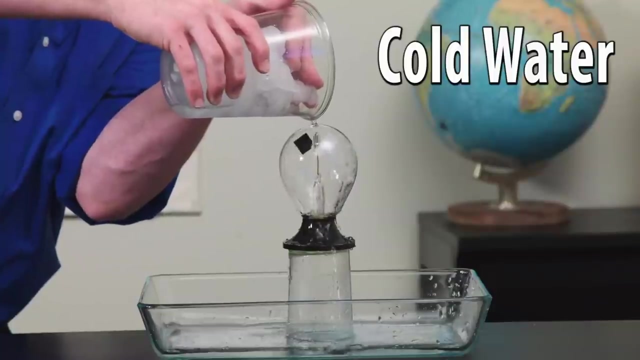 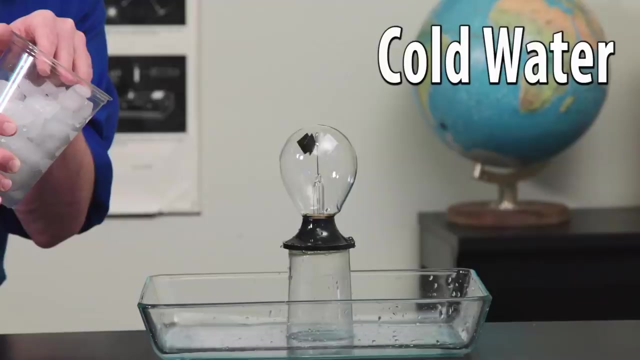 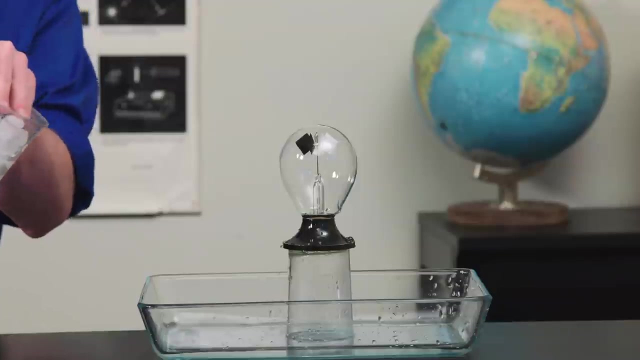 is driven not by light but by heat, and you can illustrate this by pouring some hot water on top. It begins to spin very quickly. Now watch this Cold water. Wait, Now it's spinning backwards. The explanation for this effect is found in the article linked below. 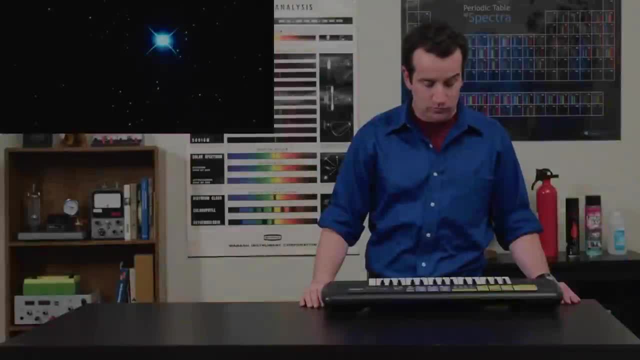 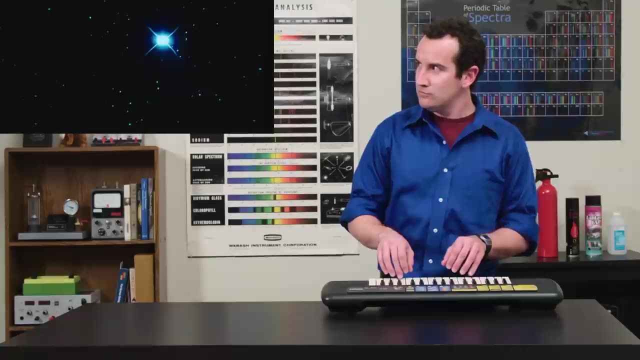 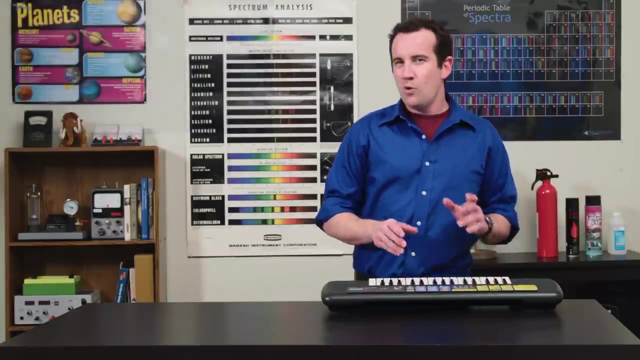 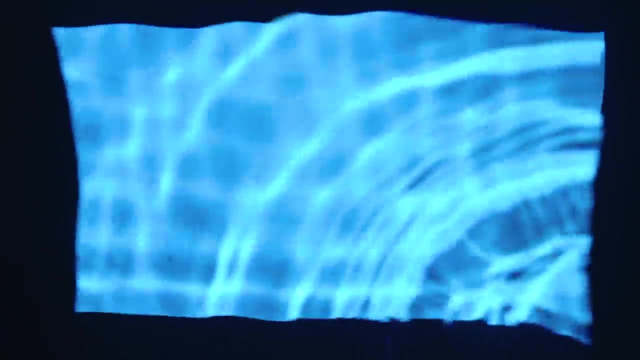 Now it's spinning backwards. The explanation for this effect is found in the article linked below. Why do stars twinkle anyway? Well, have you ever seen light rippling on the bottom of a swimming pool? The light from the stars is also rippling, but not from water, It's. 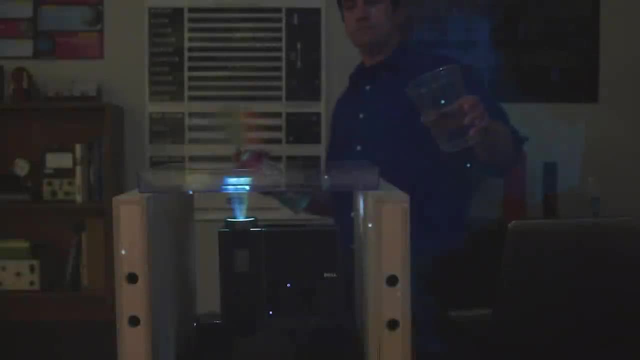 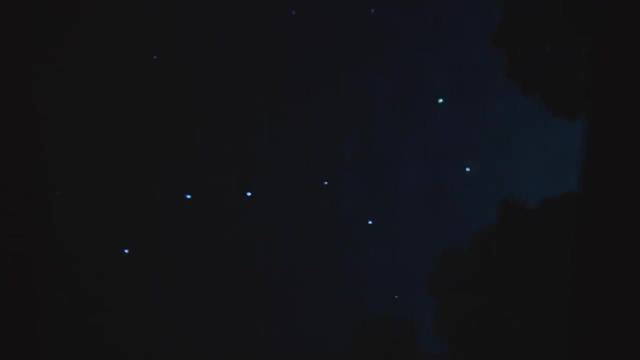 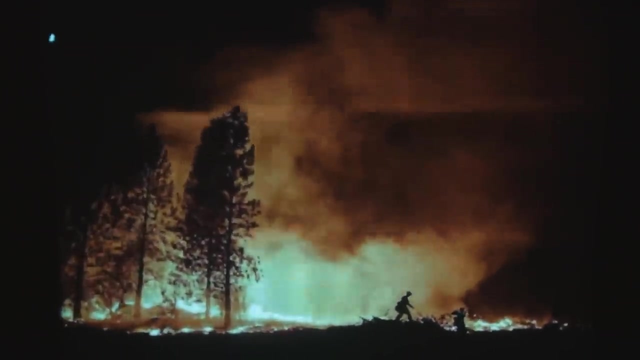 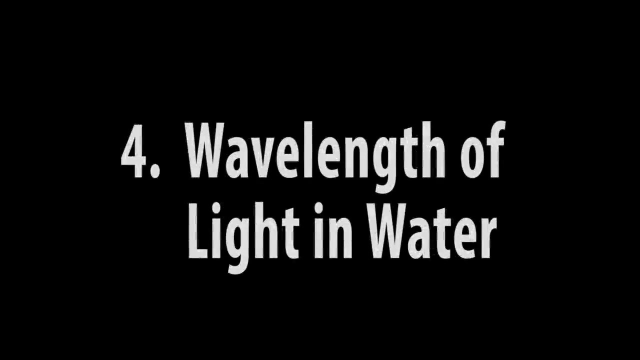 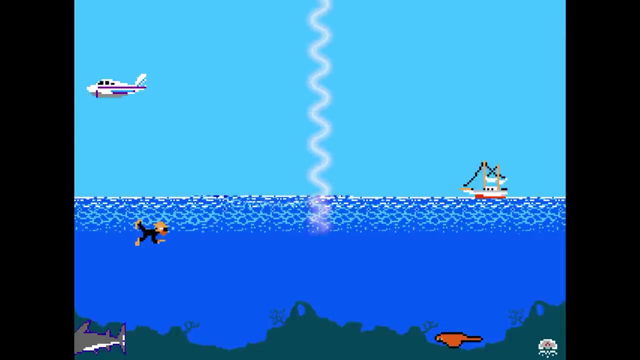 from the motion of our atmosphere. Demonstrate this by projecting a constellation through a ripple tank of water. Cause some turbulence in the atmosphere and there you go, Twinkling. What other phenomenon can you explain with this? When light travels under water, its wavelength changes. 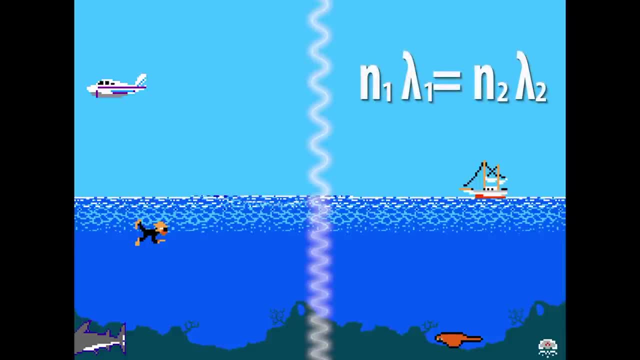 N1 lambda 1 equals N2 lambda 2.. But how could you prove this? Normally, we can measure the wavelength of light by measuring the wavelength of light. But how can you prove this? Normally, we can measure the wavelength of light by measuring the wavelength of light. 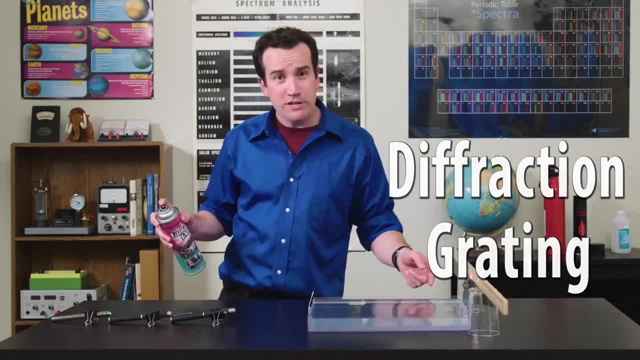 N1 lambda 1 equals N2 lambda 2.. But how could you prove this? Normally, we can measure the ausge decay of light and N2 lambda 1- equals want photovoltaics. N1 lambda 1 equals N2 lambda 2.. But how could you prove this? Normally, we can measure the. 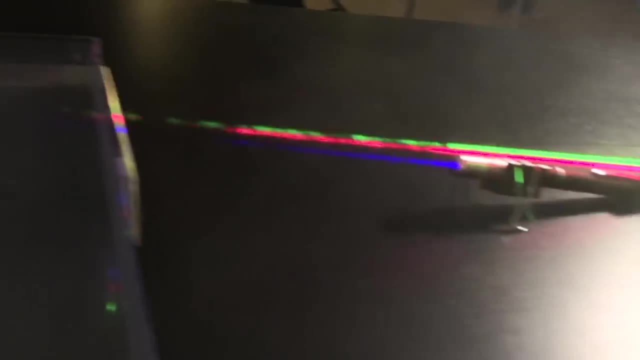 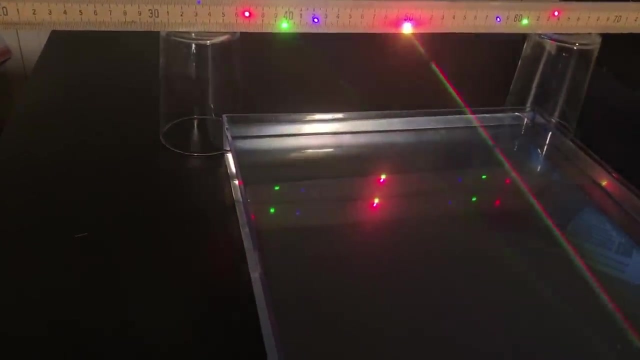 wavelength of light by measuring theidable gravity of light. So N1 lambda 1 equals N2 lambda 2 squared, or N2 lambda 1 equal to two Australenic degrees and two Kegels per second times 4 kurzur story. 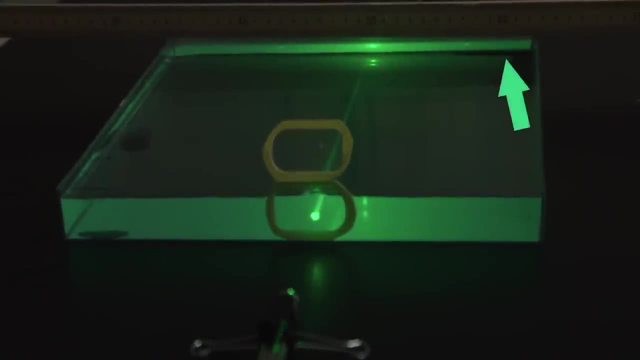 Now, if this hasn't beenätted, it'll be excluded through sort of a vers Verite. N2 delta 1 means it's less than one метrage away from the surface. perchings- the color of women, friends and the universe. modify L. 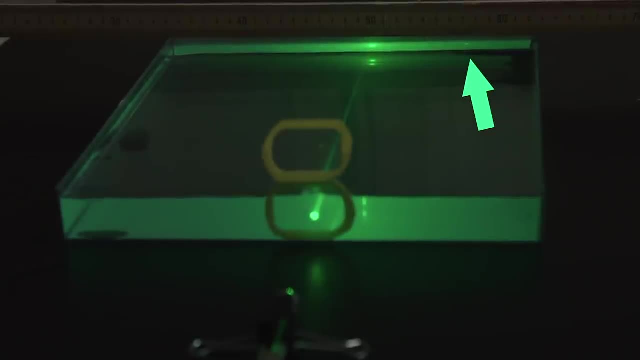 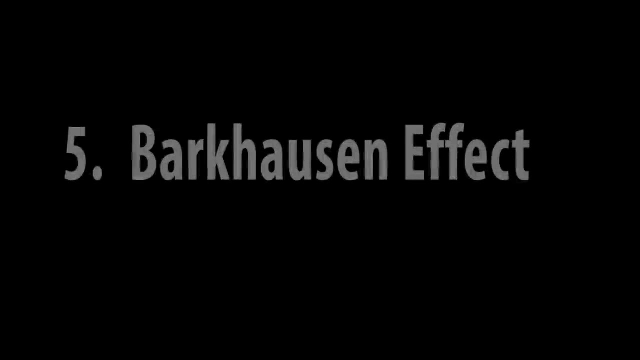 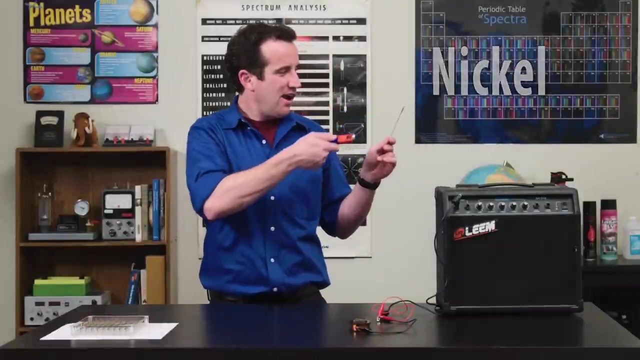 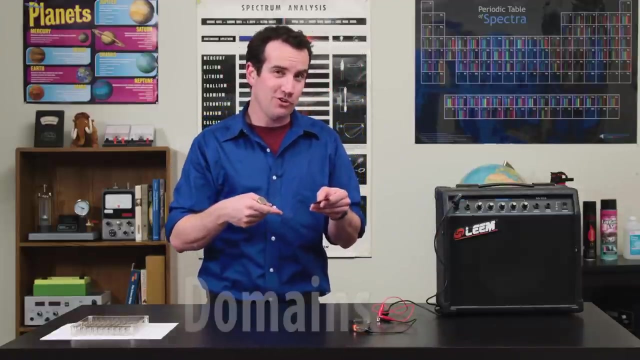 사막처럼. Was it that Hatem? It's honey and, more importantly, it's consistent with the theory. Is nickel magnetic? I guess it is. The magnetism is formed when tiny little crystals called domains. 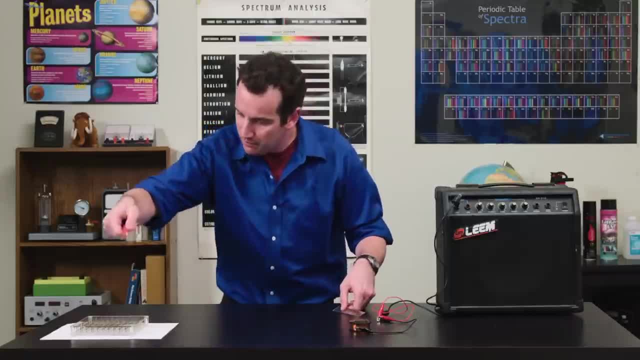 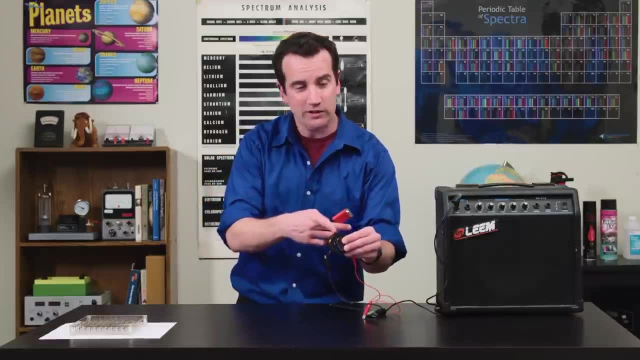 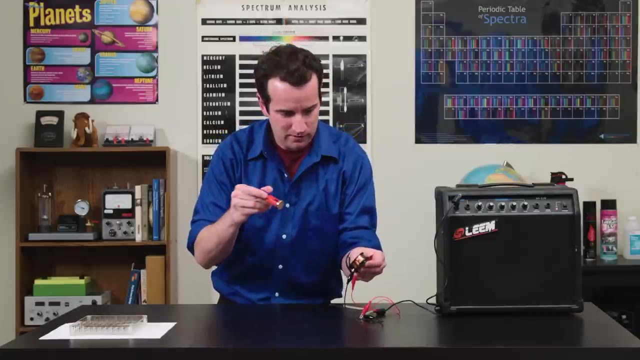 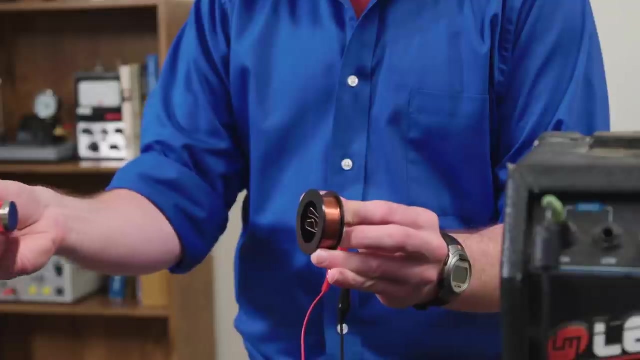 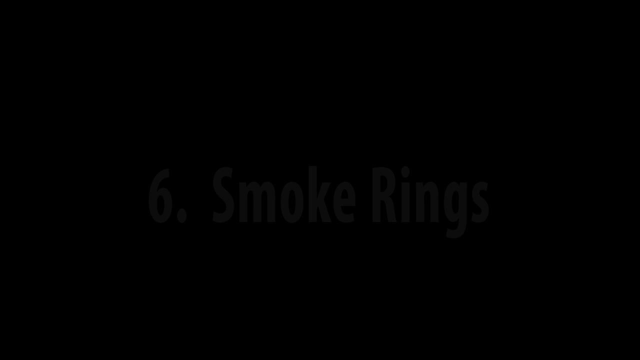 grow in the direction of the magnetic field. You can hear the magnetism taking shape. if you place the nickel in a coil that's connected to an amplifier, A crackling will be heard as the domains form. Do you hear it? You might own one of these Airzooka air cans. 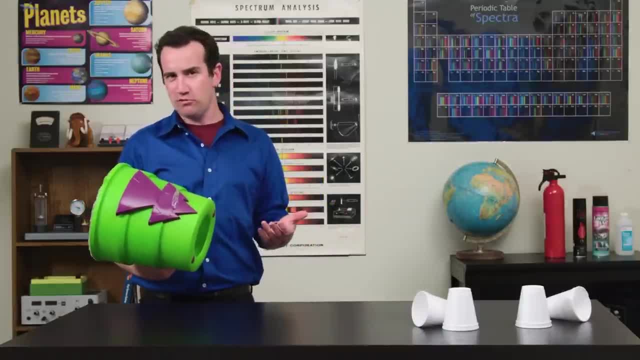 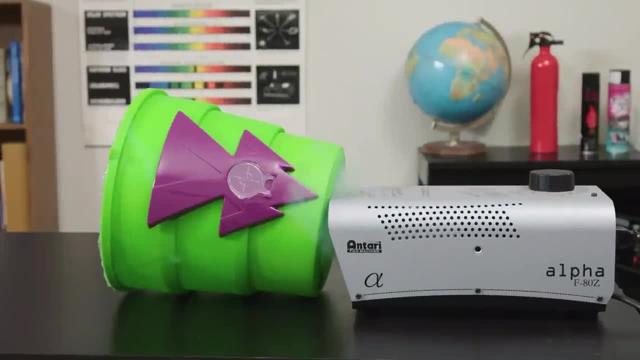 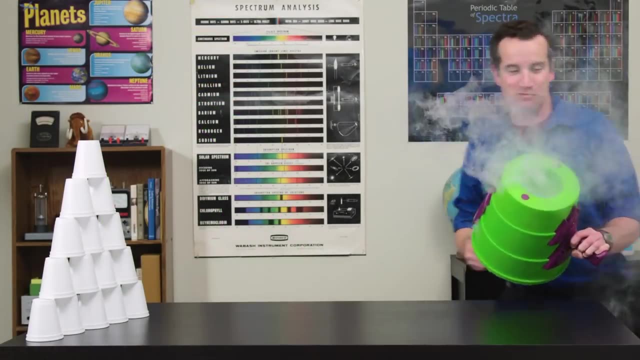 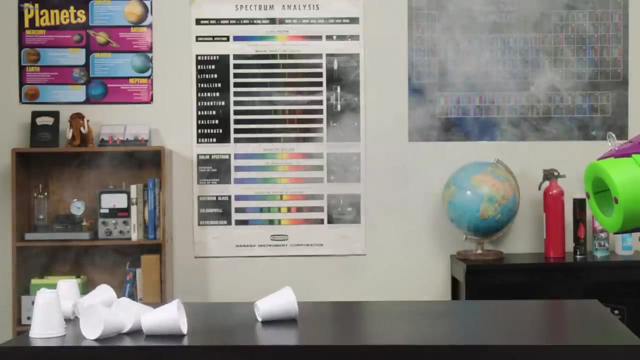 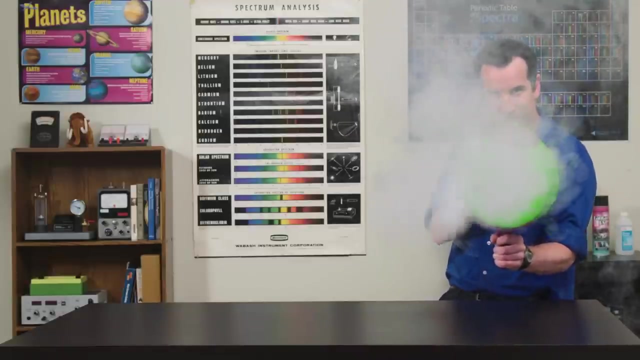 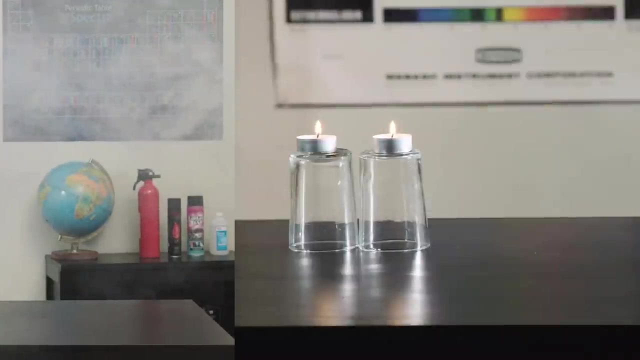 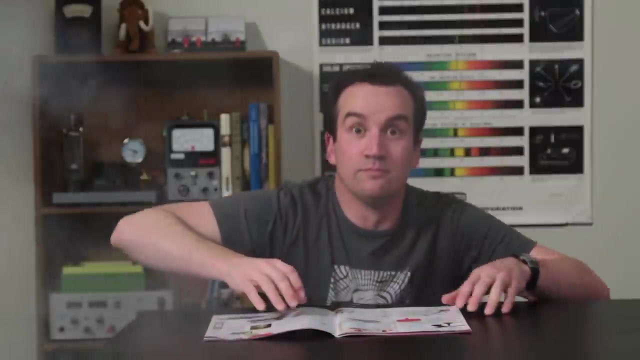 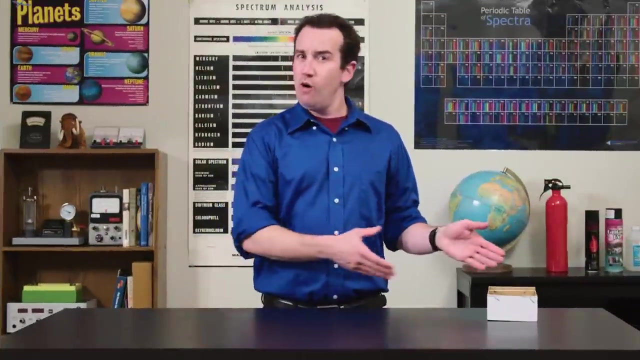 It works by shooting a vortex, which is like a smoke ring, except invisible, Unless you add smoke. Now, with smoke in place, we can actually see the vortex ring, Use it to blow out birthday candles or wake sleeping students. Do you already do this demonstration with pulling a rubber band across a box? 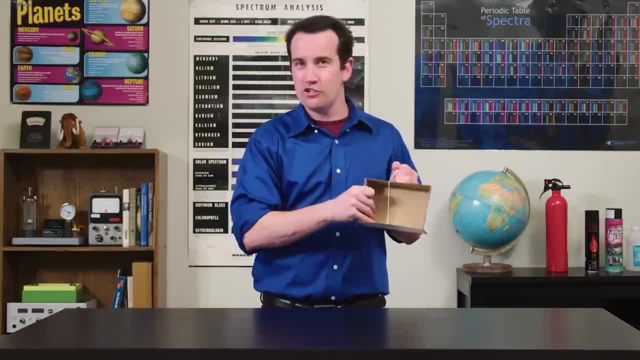 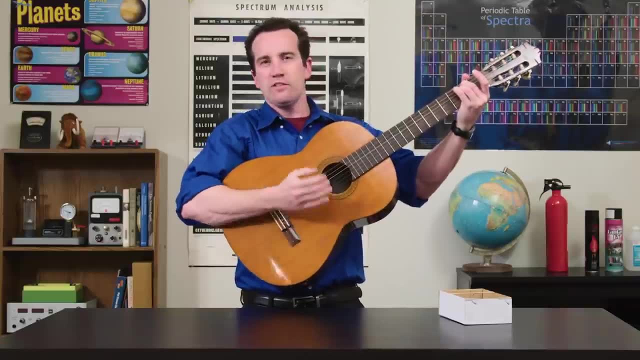 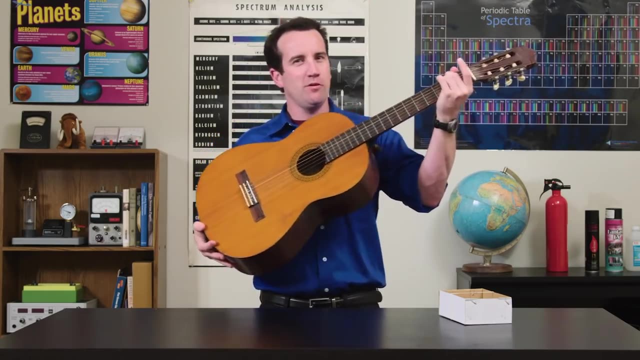 changing the tension, changing the musical note. This is similar to how a guitar works. On a guitar, the strings are pulled tight in a tension across the sounding board which vibrates, so you can hear them all much louder. But there's a better way to do this demonstration. 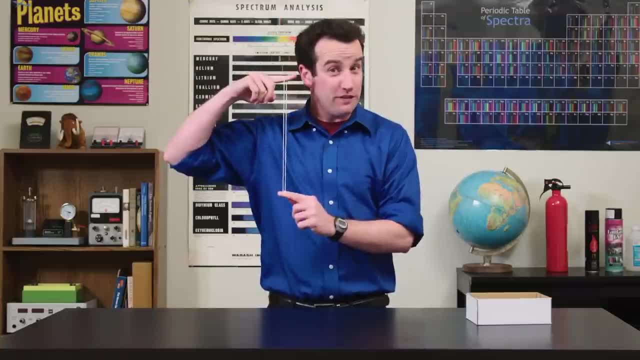 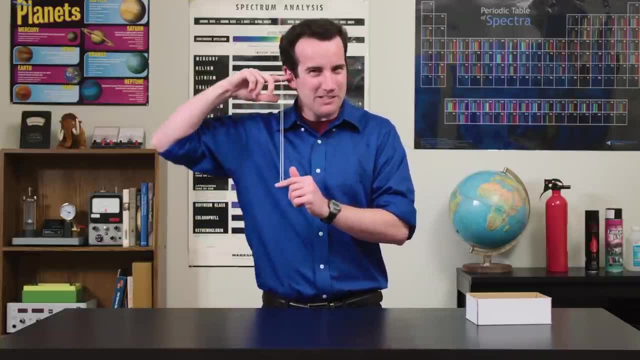 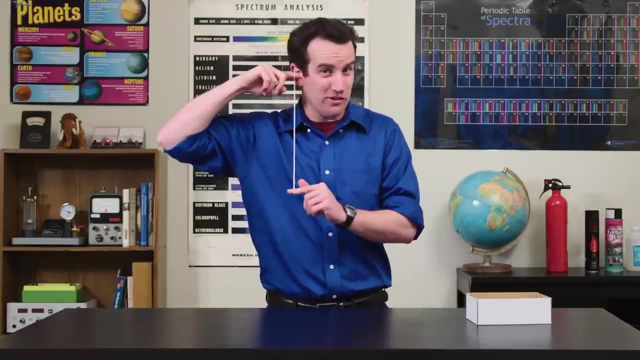 Take the rubber band and pull it and stick your finger in your ear. Now the rubber band is going to sound like a bass guitar in your head as the sound goes through your finger into your skull. And the best part is. 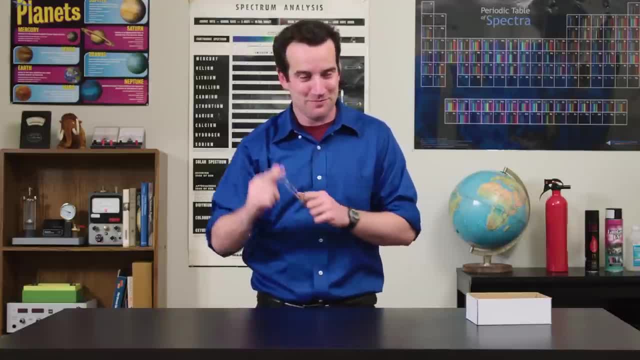 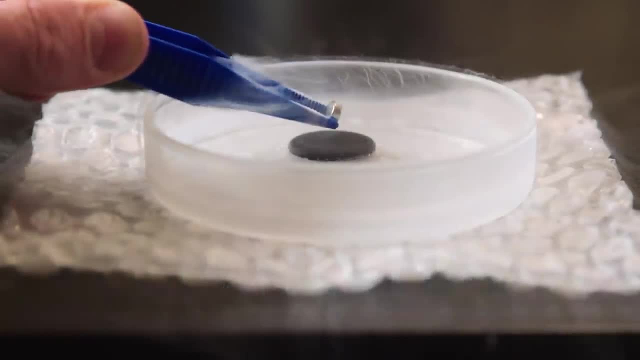 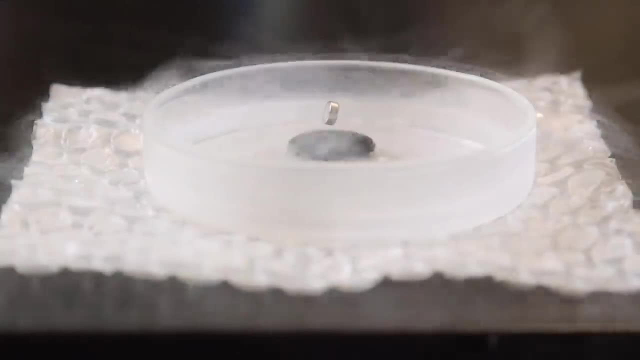 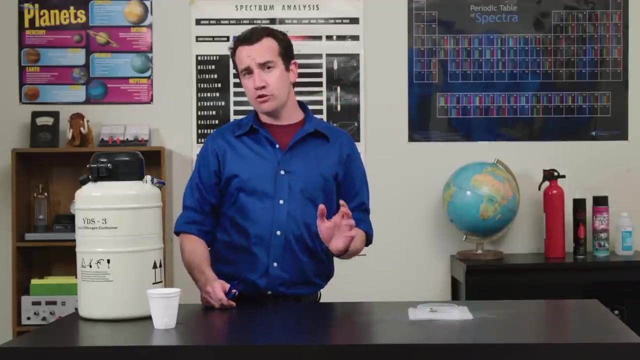 all of your students can try this at the same time. Superconductivity is already an impressive demonstration: The currents generated do not weaken with time and cause a perfect magnetic repulsion. But what most people don't show is that the superconductor is actually expelling the magnetic fields. 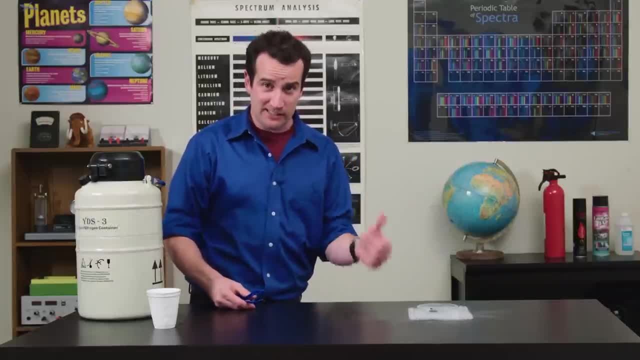 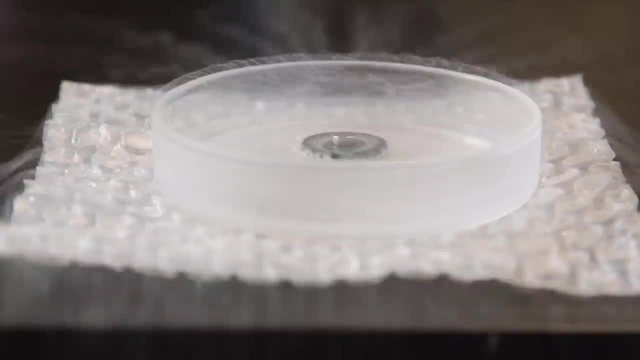 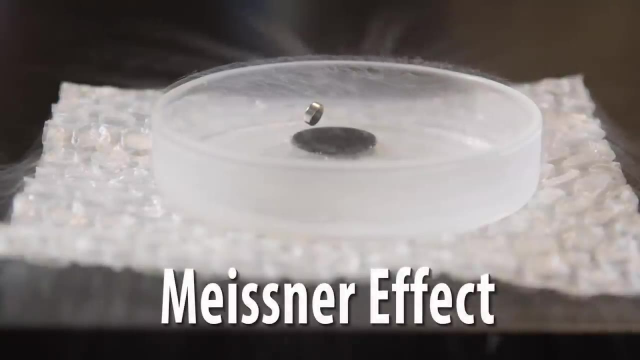 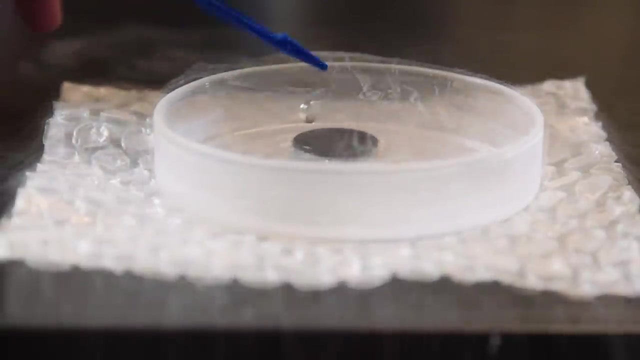 as the phase change occurs, The magnet gets lifted out. This is called the Meissner effect, The expelling of magnetic fields. The point is, superconductors are not just perfect conductors. They are a completely new phase of matter that expels magnetic fields. 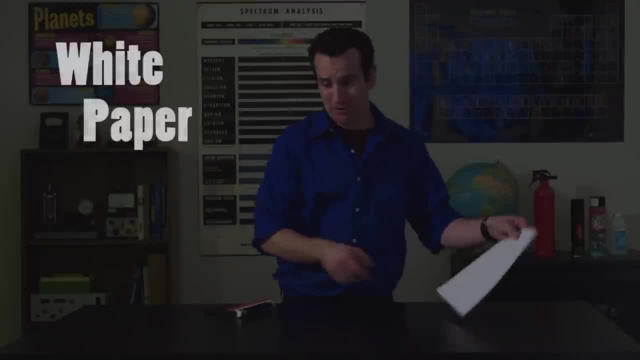 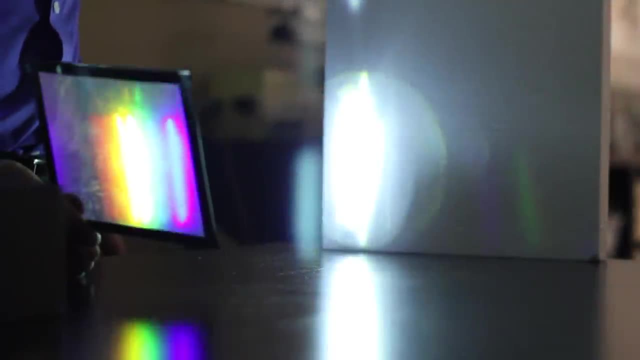 For a long time now, I've used white paper as a means by which to find ultraviolet light. Here we see the lines of the mercury spectrum, And the styrofoam does not fluoresce, so it's good to compare the two. 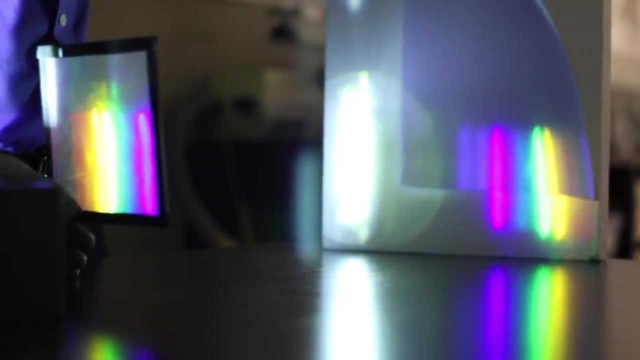 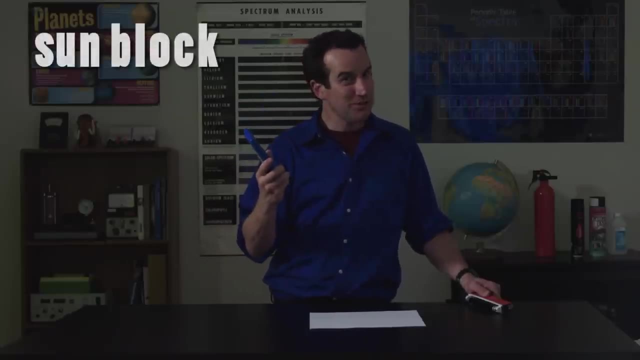 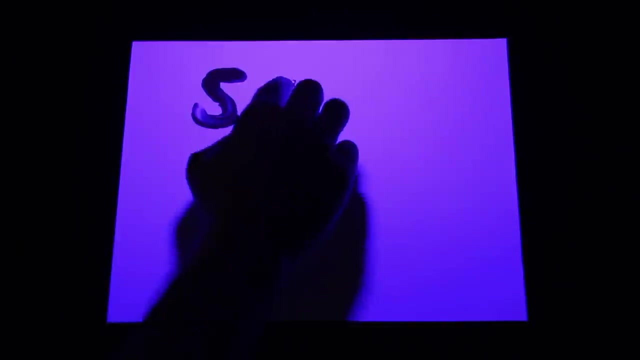 and dramatize the situation. I will now use this approach to test out how effective sunblock is. What is sunblock supposed to do? Block ultraviolet light? Here we go. Yes, The white lotion appears dark in the ultraviolet. 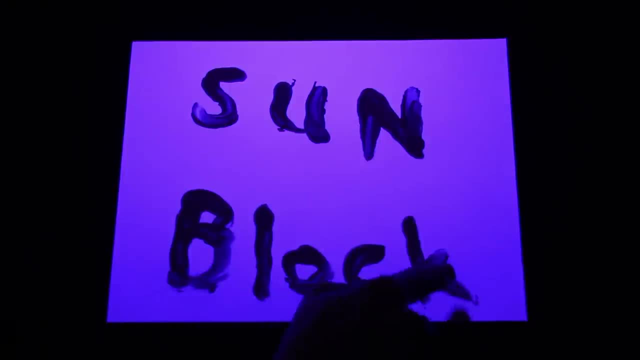 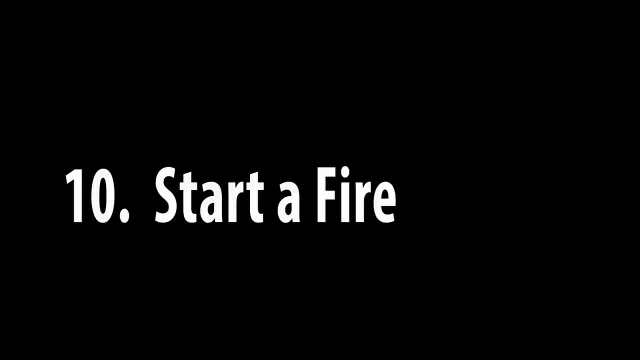 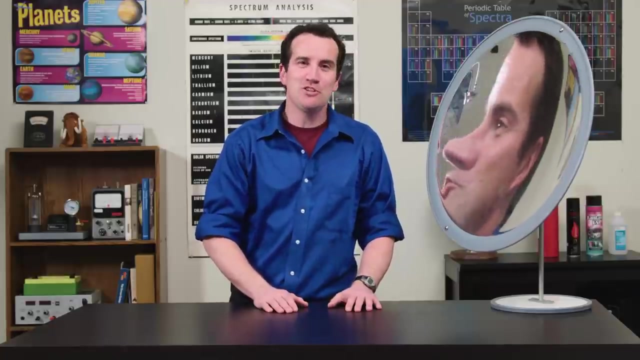 I hope your students will be convinced that this stuff really works and that they should use it. This concave mega mirror can make a lot of funny images And it's similar to those used by telescopes to focus light. The focal point is half the radius. 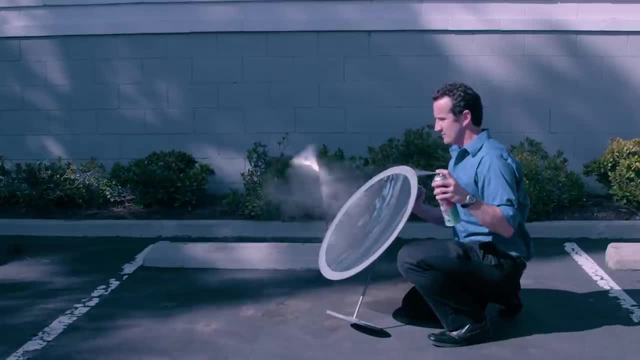 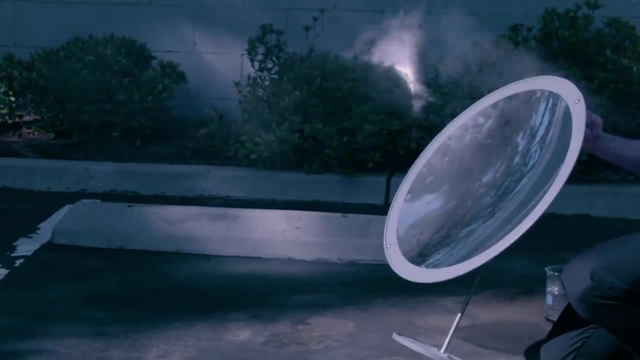 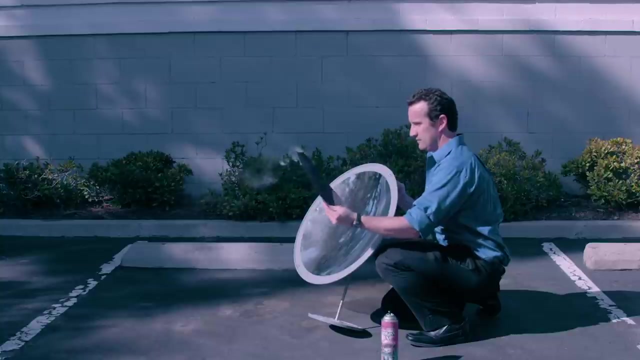 You can make this focal point visible by using fog in a can. outside on a sunny day, The focus is clearly visible when facing the mirror toward the sun and spraying the fog. Place a bit of dark construction paper at this point and it will immediately burst into flame.